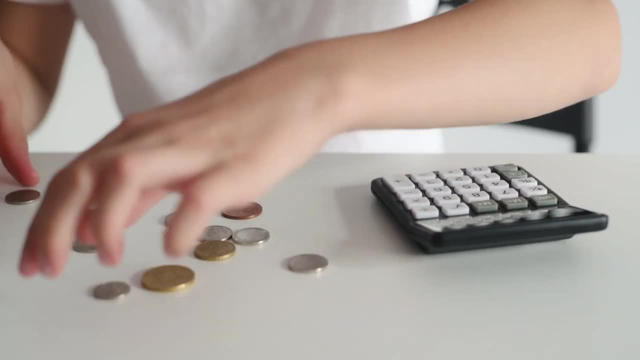 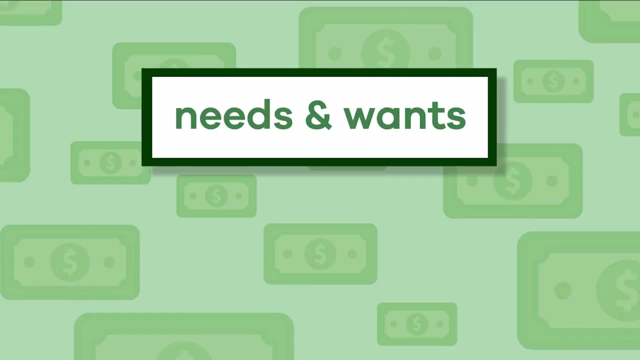 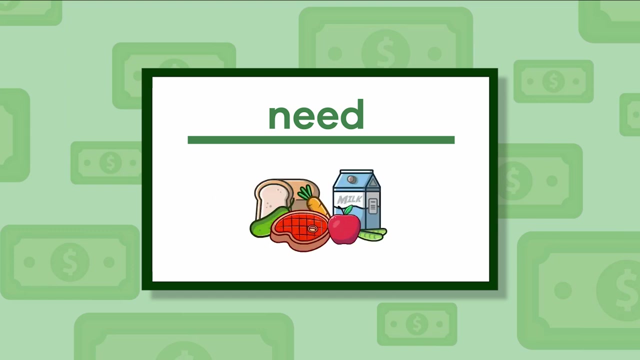 that will help you become more financially literate. Let's grab our friend Frankie Finance to help us along the way. Needs and Wants. A need is something you must have to survive, like food, water, clothing and shelter. A want, on the other hand, 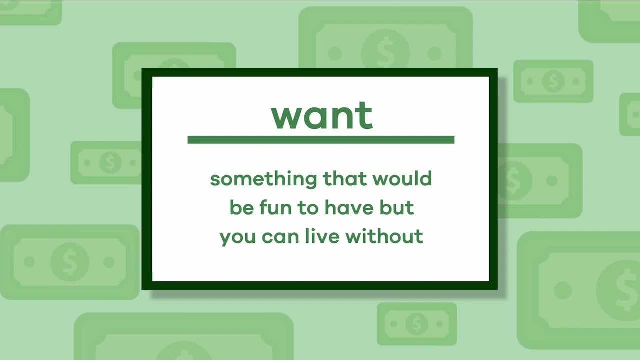 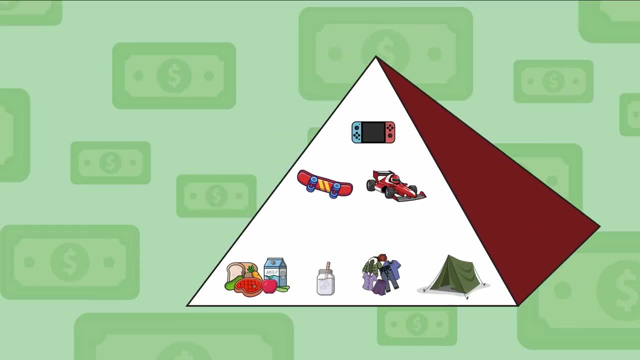 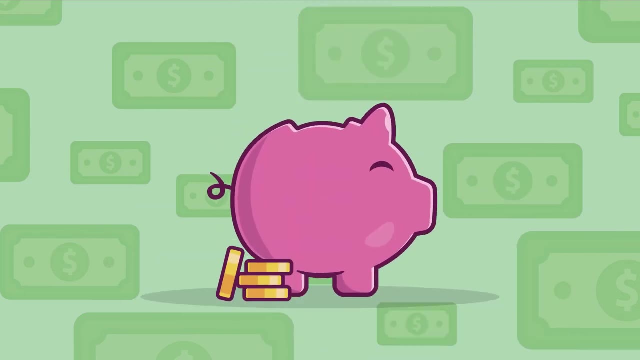 is something that would be fun to have, but you can live without, You know, like a skateboard, video game or favorite toy. Knowing the difference between needs and wants can help you be more responsible with your money, Making a Budget. A budget is a plan for managing your money. 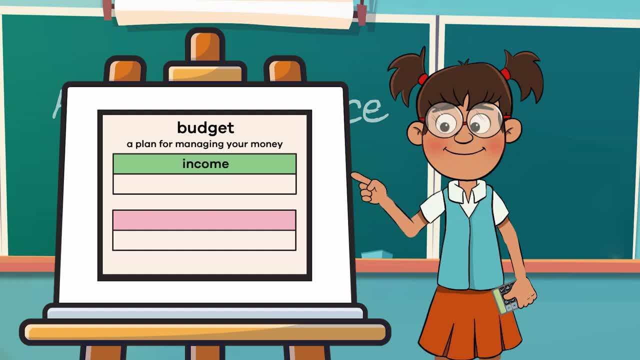 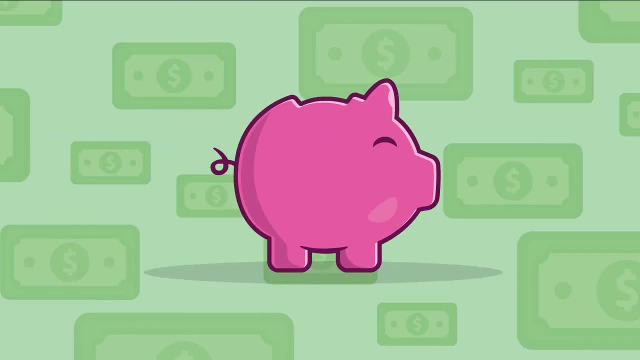 It is based on your estimation of income: the money you earn or receive as a gift, plus your expenses, meaning the money you spend. One of the main reasons to create a budget is to help you live within your means, In other words. 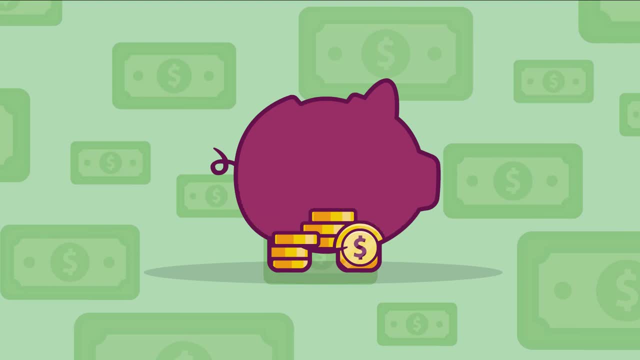 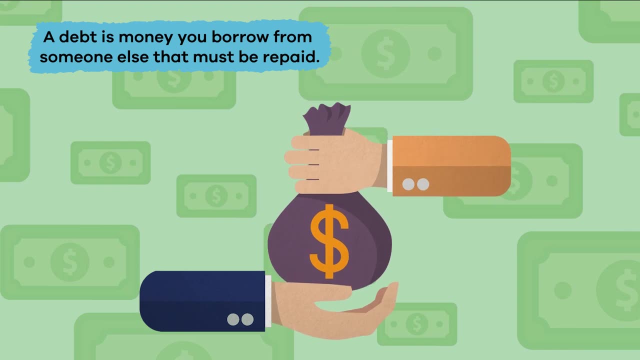 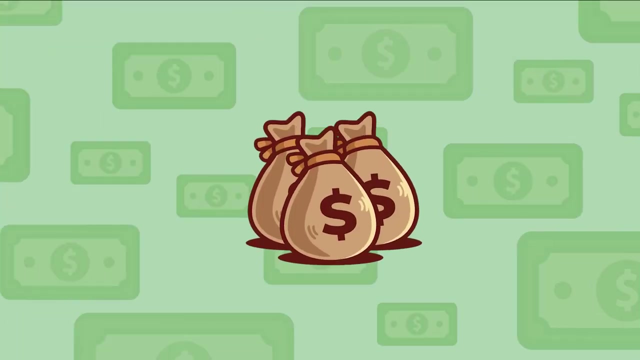 a budget can keep you from spending money you don't have and avoid going into debt. A debt is money you borrow from someone else that must be repaid. Saving vs Borrowing. Saving vs Borrowing: As you can imagine, you can probably guess. 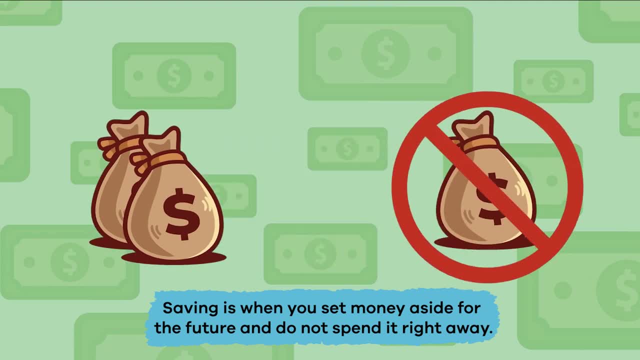 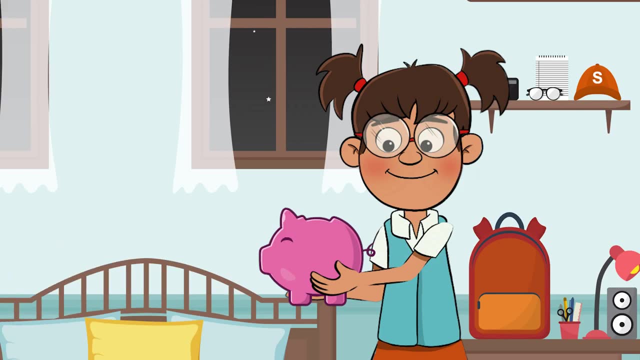 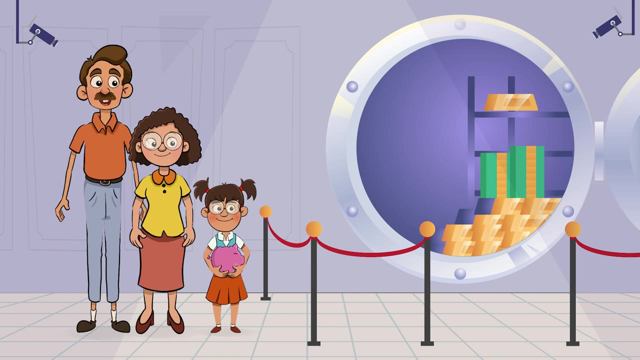 saving is when you set money aside for the future and do not spend it right away, Like if you are saving up for a special toy or activity. You might have a piggy bank at home where you put money that you are saving, Or you might even have a savings account at a bank. 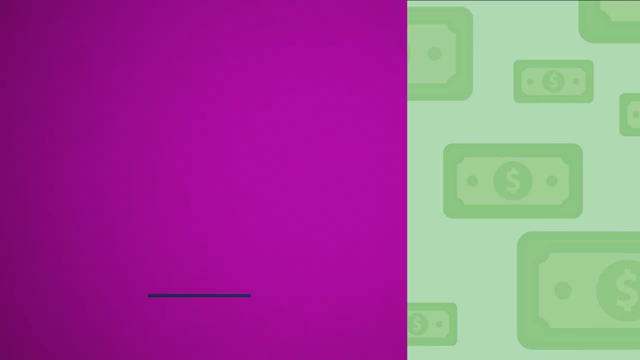 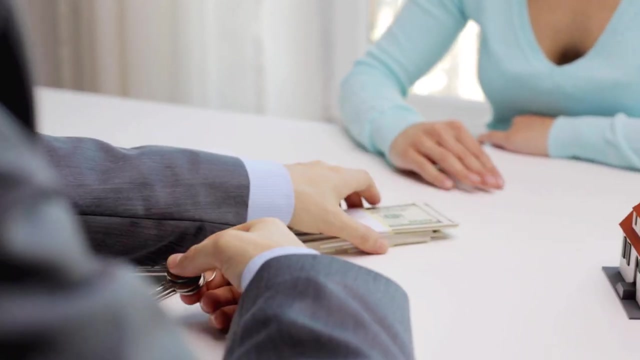 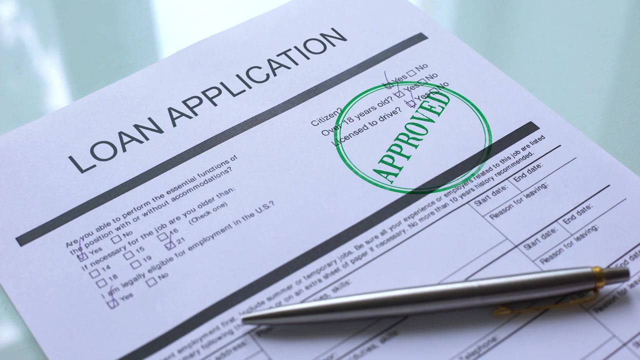 Have you ever heard of a loan before? A loan is money you borrow from someone. Borrowing money means that you are expected to pay it back. Most often, a loan is given for a specific reason, like to help purchase something big like a house or a car. 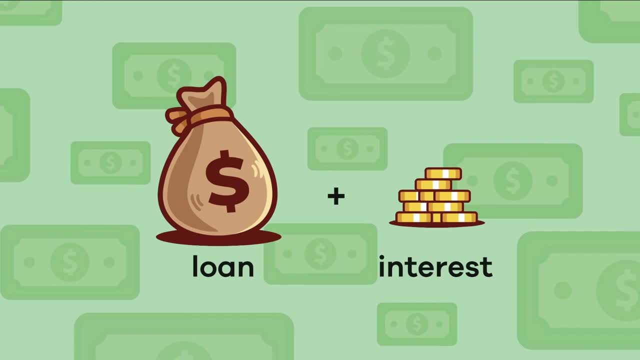 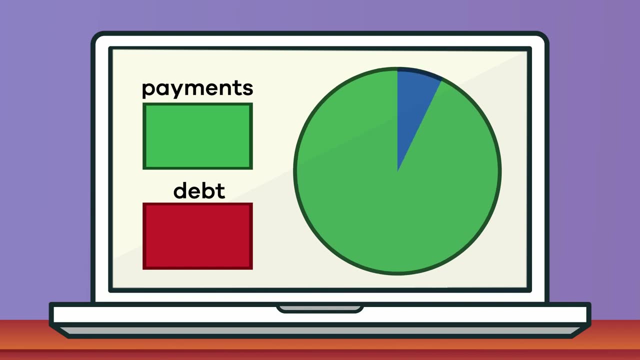 Quite often you will have to pay interest on the loan. This means the bank expects you to pay the full amount back, plus an extra charge for borrowing the money in the first place. This extra is called interest and is a huge part of our life. 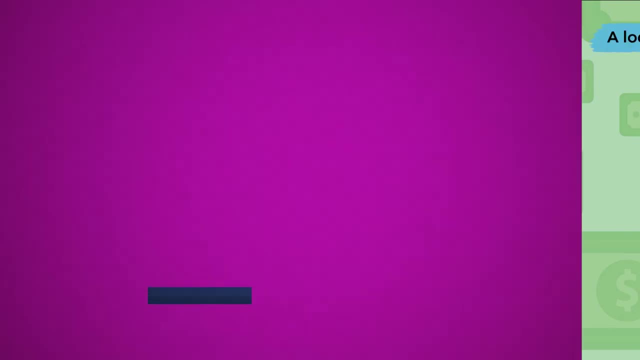 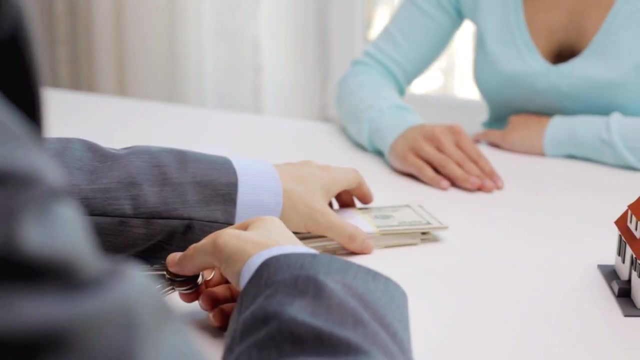 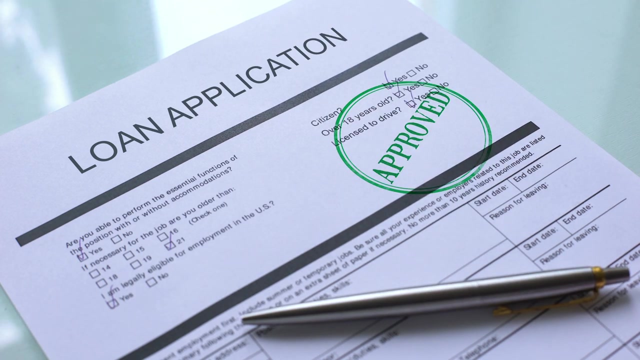 Have you ever heard of a loan before? A loan is money you borrow from someone. Borrowing money means that you are expected to pay it back. Most often, a loan is given for a specific reason, like to help purchase something big like a house or a car. Quite often you will. 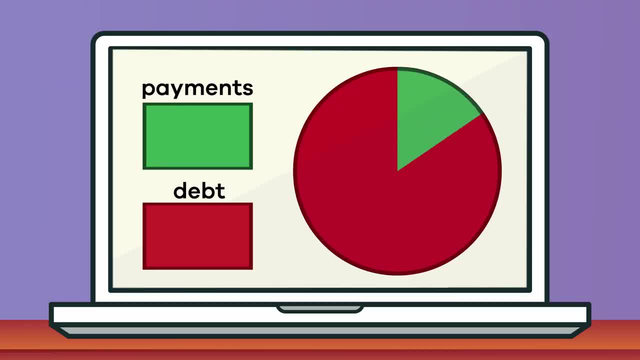 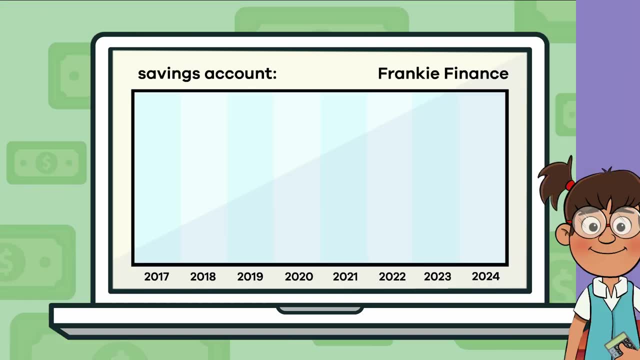 have to pay interest on the loan. This means the bank expects you to pay the full amount back, plus an extra charge for borrowing the money in the first place. This extra is called interest and is a percent of the borrowed amount. A savings account is a place where you put money. 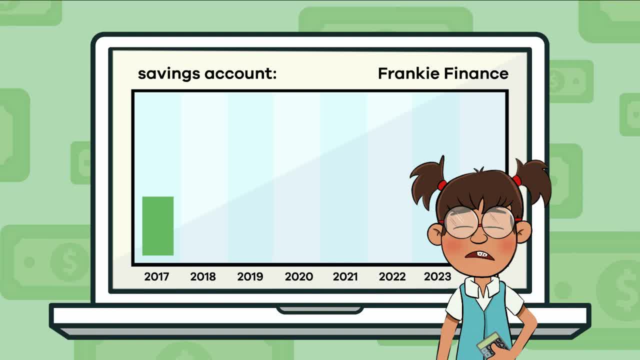 that you intend on saving for a while. And guess what? You can actually earn a little extra money while your money is in the bank. For real, This is also called interest. but instead of giving money back to the bank for a loan, it is a little extra money that you earn while your money sits. 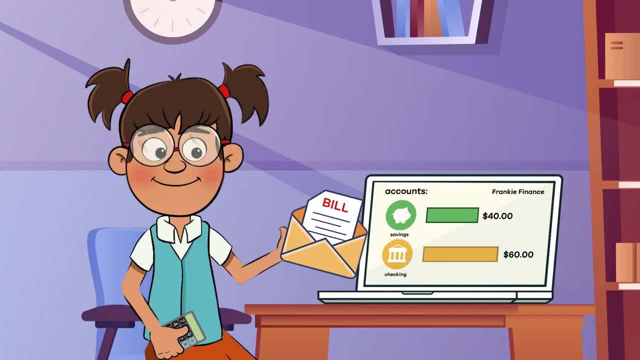 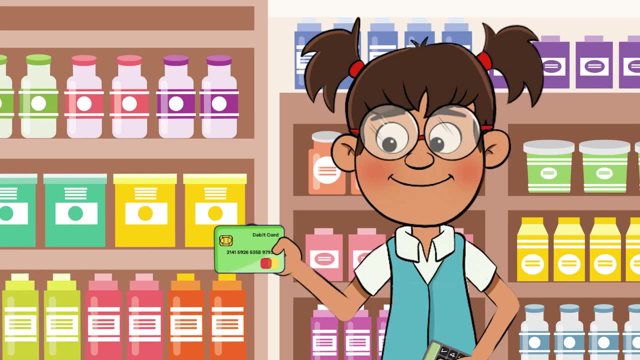 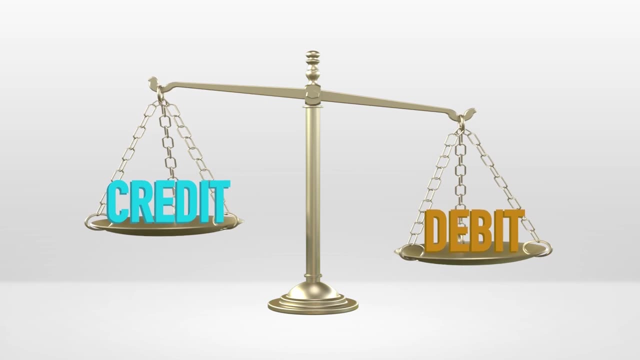 in the bank. A checking account is another kind of bank account that you can use to pay bills, either by check or by a special card called a debit card. Checking accounts do not earn interest. Credit vs Debit: A credit card is a small 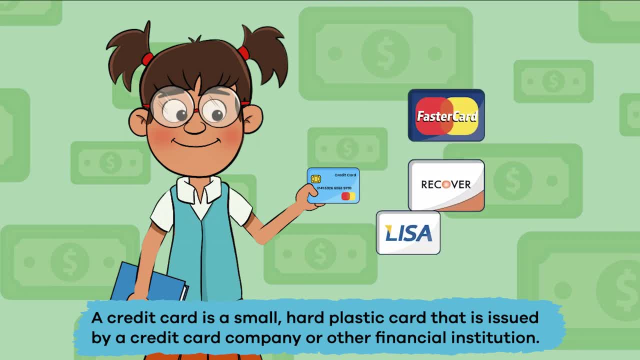 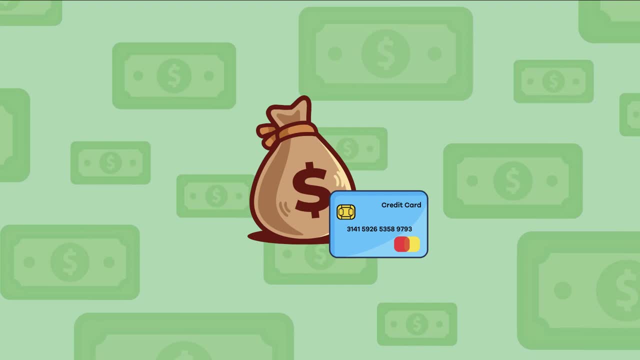 hard plastic card that is issued by a credit card company or other financial institution. They are basically a type of loan, because using a credit card means you are borrowing money from the company who issued the card. Here's how it works: The credit card company loans you money and you pay it back. 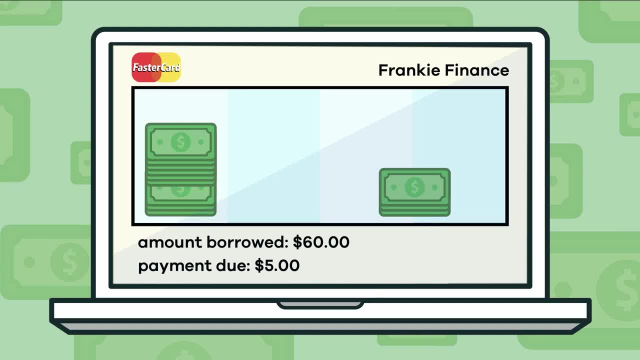 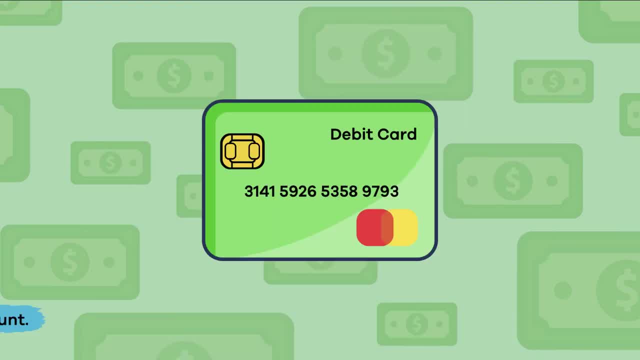 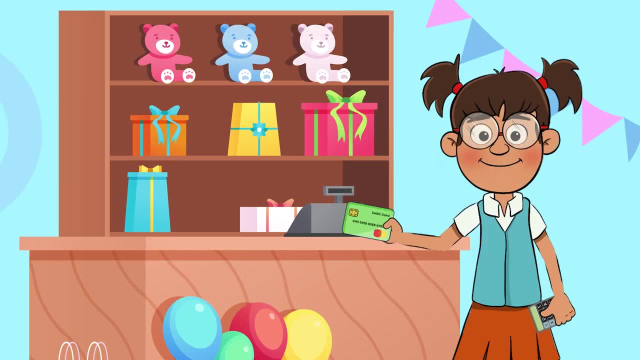 according to a schedule. This is usually one payment per month, with interest on the unpaid amount. On the other hand, debit cards are linked directly to your bank account, Which means you use your debit card to pay for things with money you already have. 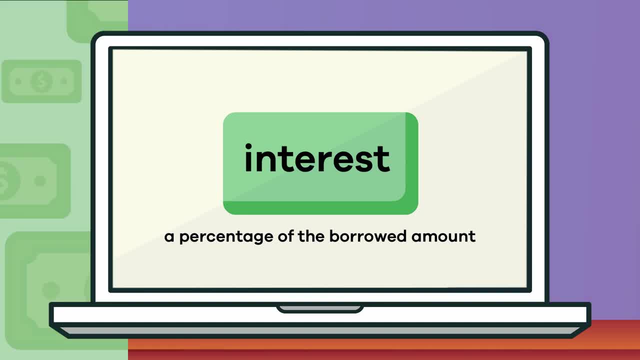 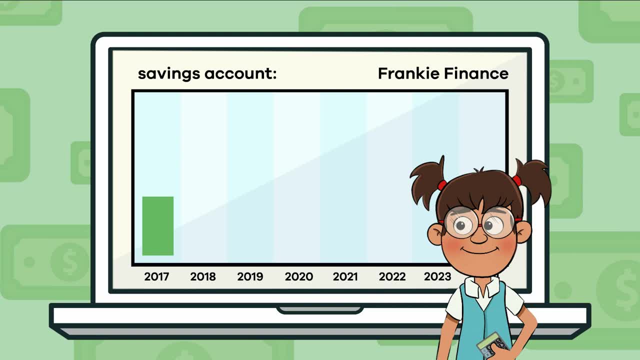 and is a percent of the borrowed amount. A savings account is a place where you put money that you intend on saving for a while And guess what? You can actually earn a little extra money while your money is in the bank. For real, This is also called interest, But instead of giving. 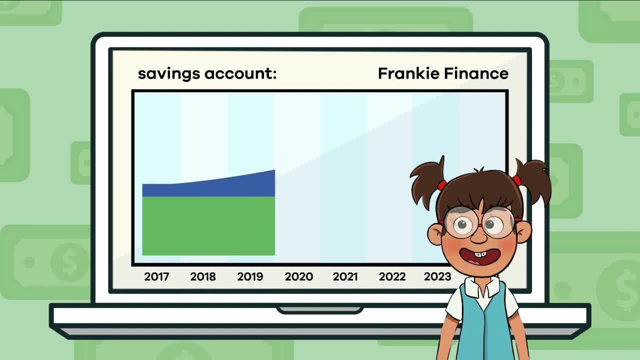 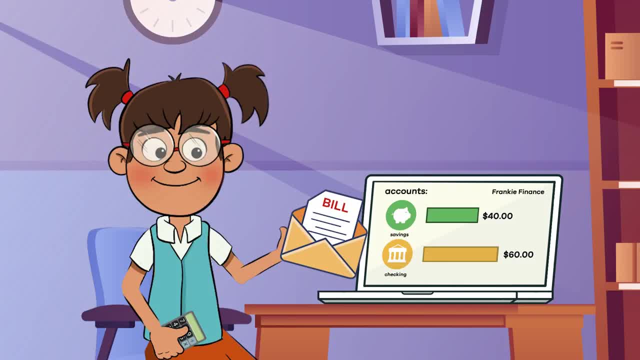 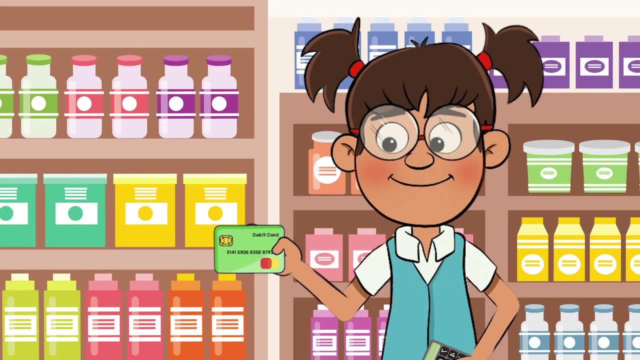 money back to the bank for a loan. it is a little extra money that you earn while your money sits in the bank. A checking account is another kind of bank account that you can use to pay bills, either by check or by a special card called a debit card. Checking accounts do not earn interest. 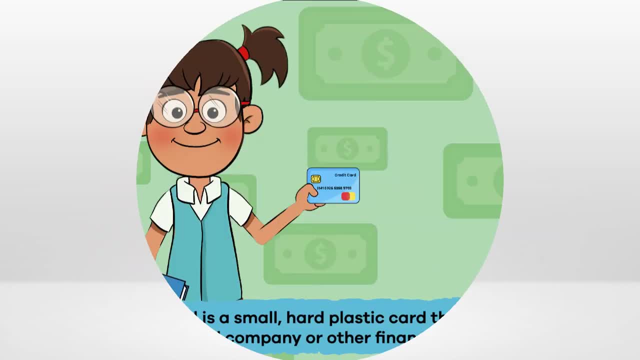 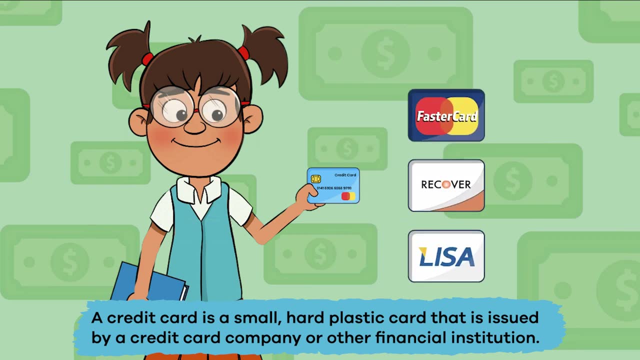 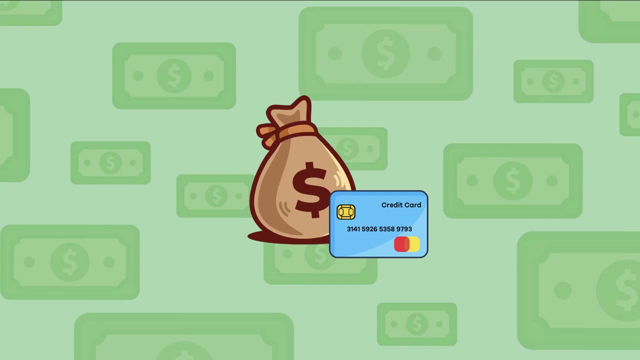 Credit versus debit. A credit card is a small, hard plastic card that is issued by a credit card company or other financial institution. They are basically a type of loan, Because using a credit card means you are borrowing money from the company who issued the card. Here's how it works: The credit card company. 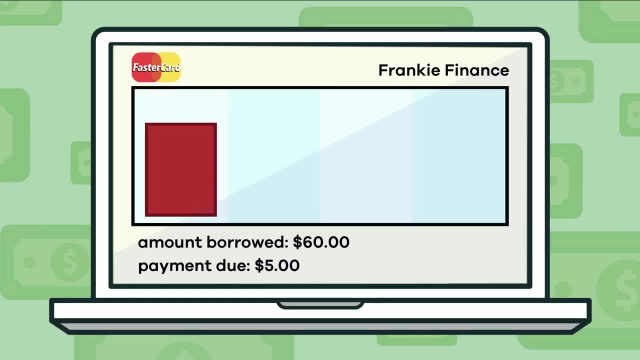 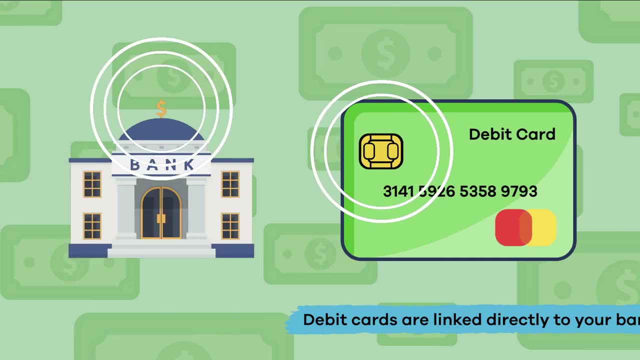 loans you money and you pay it back according to a schedule. This is usually one payment per month, with interest on the unpaid amount. On the other hand, debit cards are linked directly to your bank account, Which means you use your debit card to pay for things with. 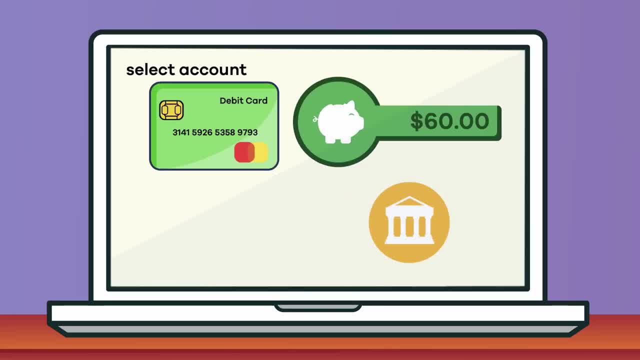 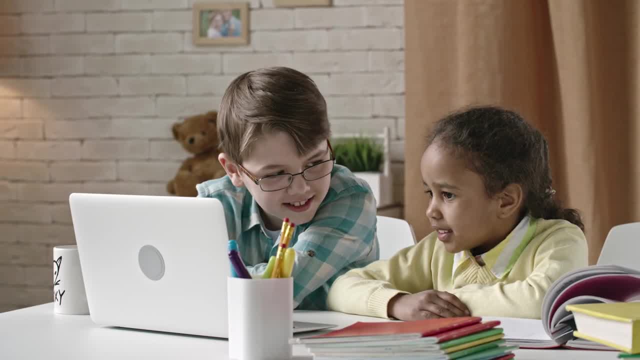 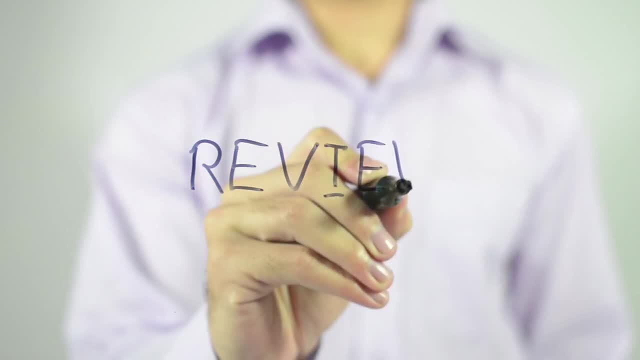 money you already have in either your savings or checking account. Want to learn more? We have more videos that go into more detail about each of these skills. For now, let's review what we learned today. True or False, Checking and savings accounts are. 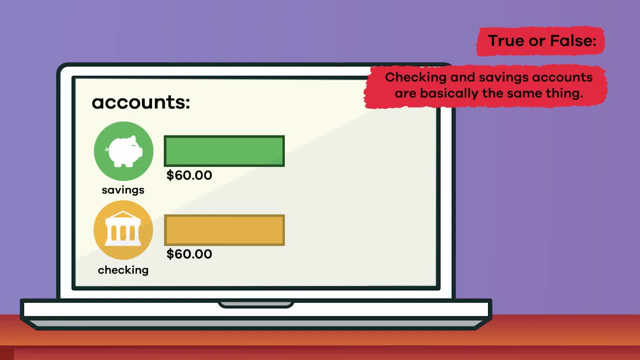 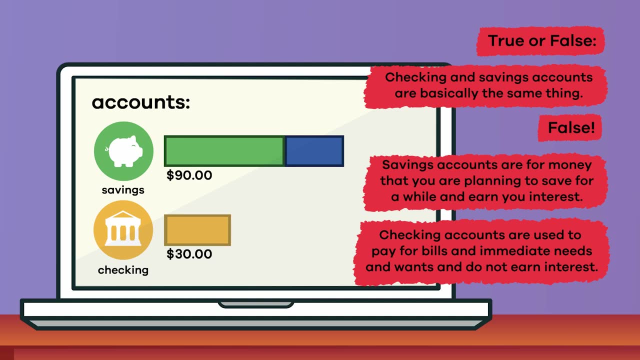 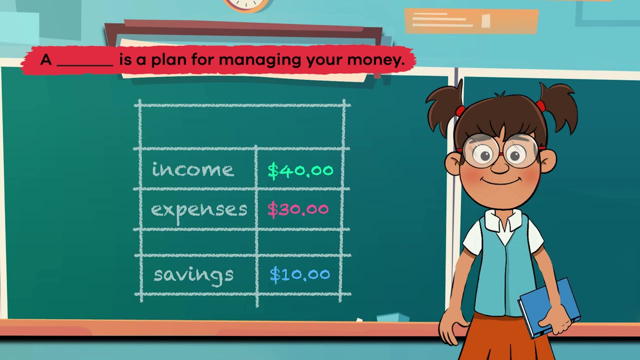 basically the same exact thing. False Savings accounts are for money that you are planning to save for a while and earn you interest. Checking accounts are used to pay for bills and other immediate needs and wants that do not earn interest. Fill in the blank. A blank is a plan for. 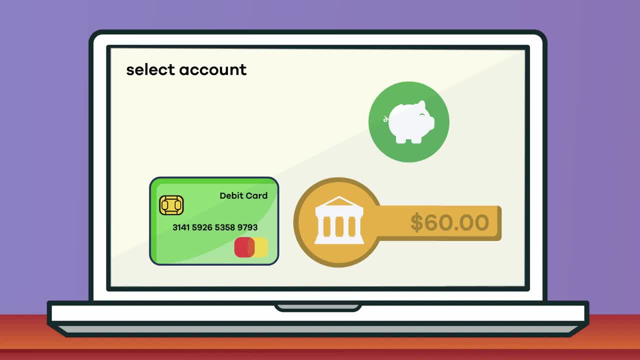 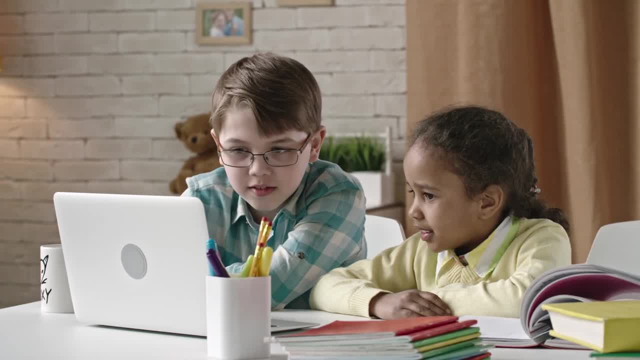 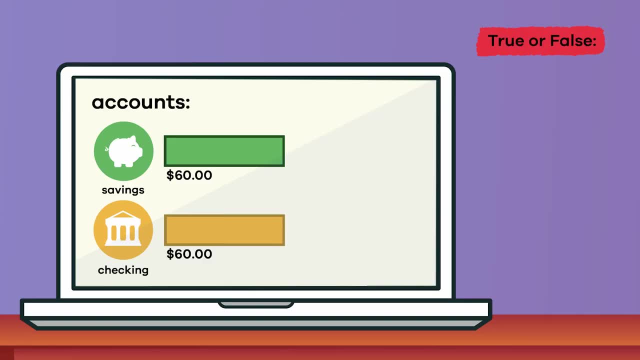 in either your savings or checking account. Want to learn more? We have more videos that go into more detail about each of these skills. For now, let's review what we learned today. True or False, Checking and savings accounts are basically the same exact thing. 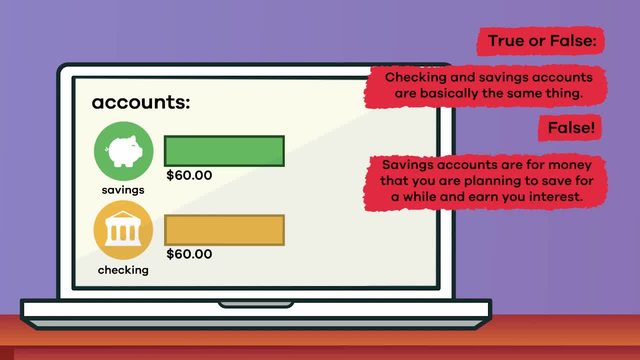 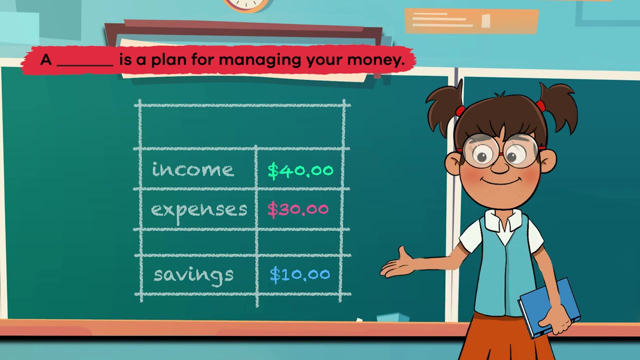 false. Saving accounts are for money you are planning to save for a while and earn you interest. Checking accounts are used to pay for bills and other immediate needs and wants that do not earn interest. fill in the blank. A is a plan for managing your money. 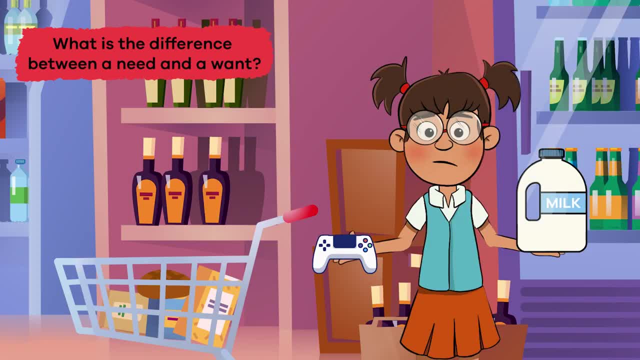 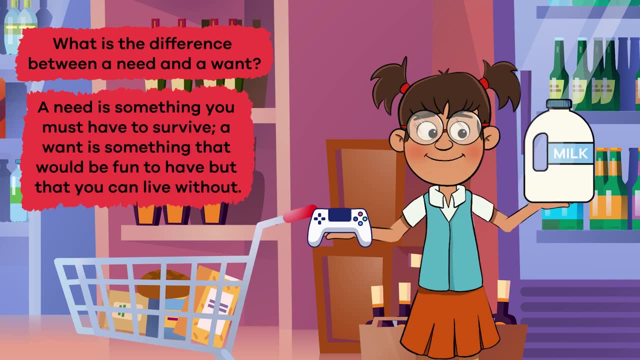 budget. What is the difference between a moneyand interest Banking? is a Online bankCHECKING counts a market cap: rho- ordinate dollarsR. Growth Bank is an emotions index that doesn't handle financial unable. a need and a want. A need is something you must have to survive. A want is something that would 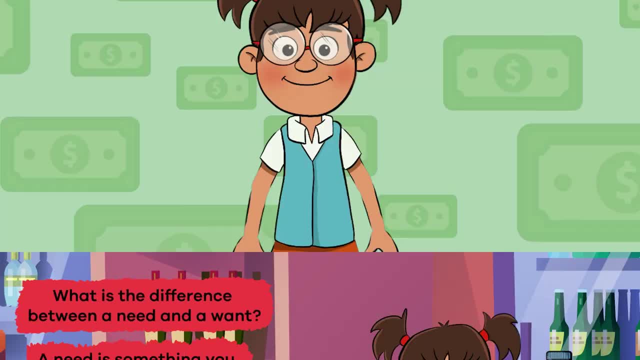 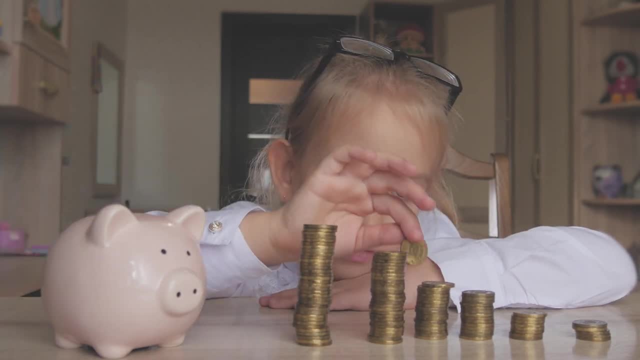 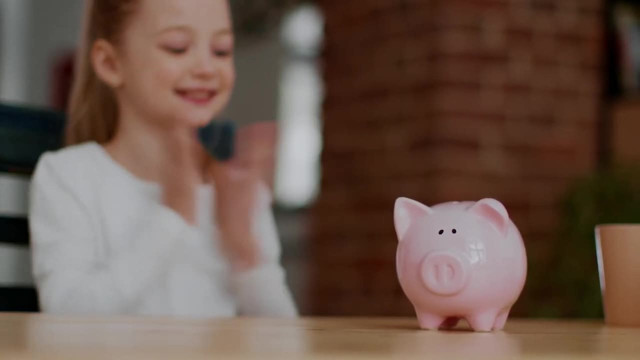 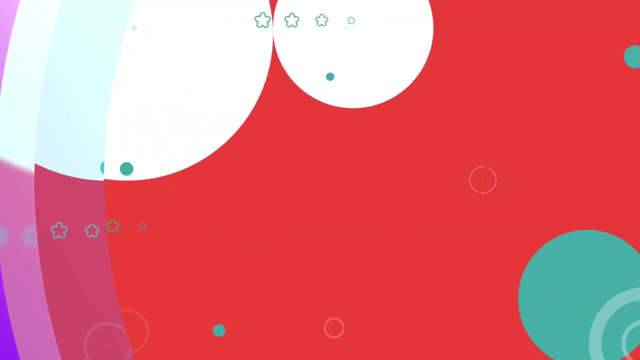 be fun to have, but you can live without Fantastic job, financial friends. Learning financial literacy is important as you create good money habits for the future. What is one thing you can work on to become more financially literate? Hope you had fun learning with us. Visit us at LearnBrightorg for thousands of free resources. 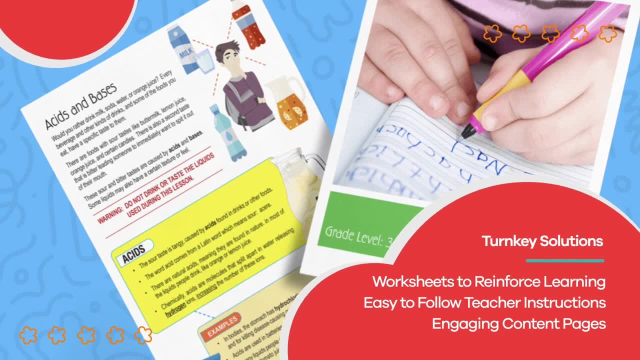 and turnkey solutions for teachers and homeschoolers. 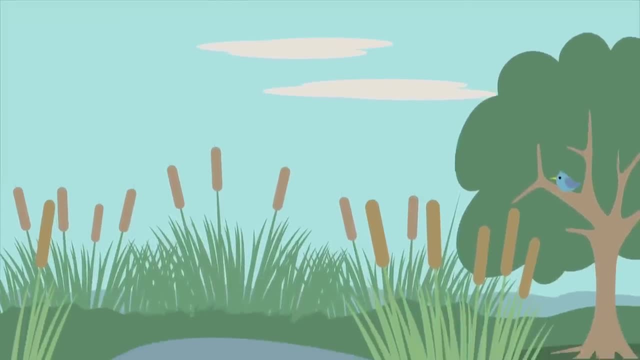 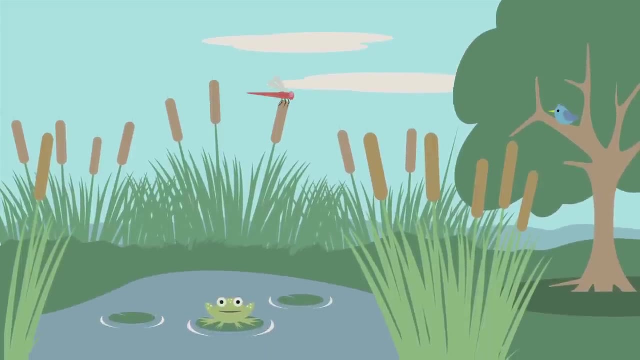 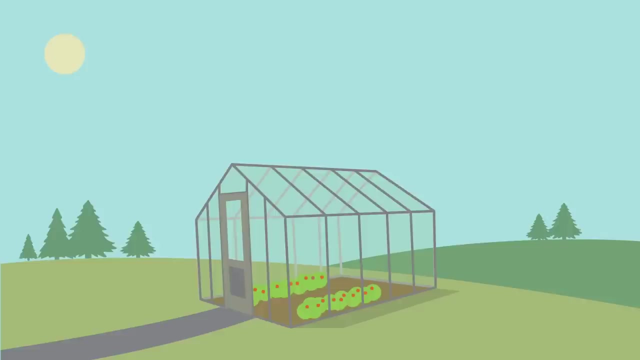 What is the greenhouse effect? Earth is a comfortable place for living things. It's just the right temperature for plants and animals, including humans, to thrive. Why is Earth so special? Well, one reason is the greenhouse effect. A greenhouse is a building with glass walls and a glass roof. The clear glass allows